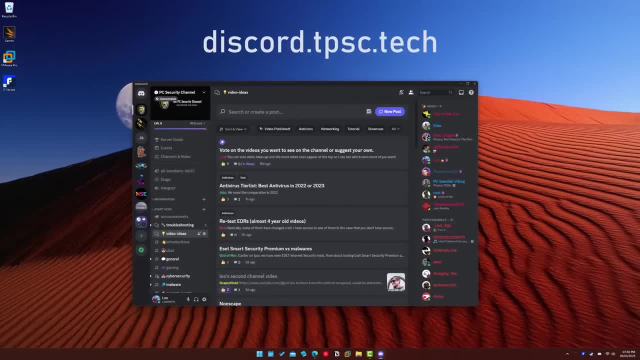 and some intelligent automation. Before we get started, I just wanted to announce that we'll be doing a custom workshop event for this video, So if you want to join that, check out the link in description to join our Discord. It's a great way to hang out with the community. I'll be there. 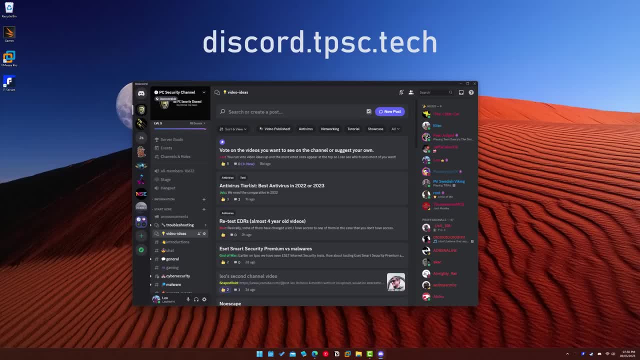 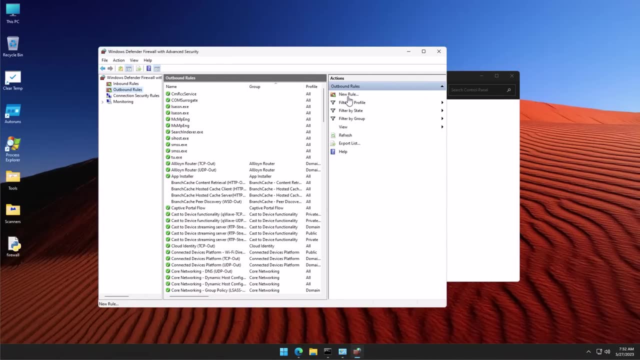 of course, You can ask any questions. We'll have fun, maybe even play some games. So if that's your kind of thing, join the Discord. In order to do this, we're going to use Windows Firewall's ability to create rules Now using the GUI. it's pretty straightforward, You. 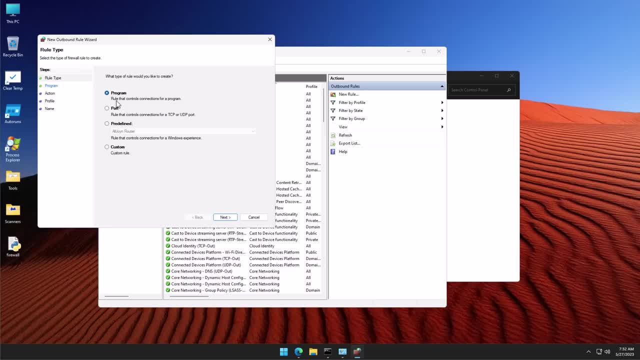 can select any type of rule. So, for example, if you want to filter a specific program, you select program. If you want to block a port, you select port, predefined or custom- We're going to go custom. And then essentially what we want to do is for all programs blacklist a specific remote. 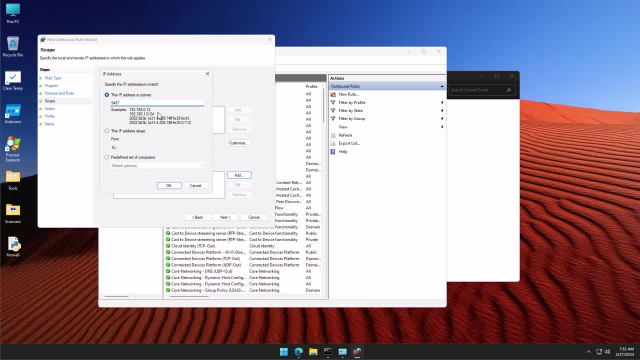 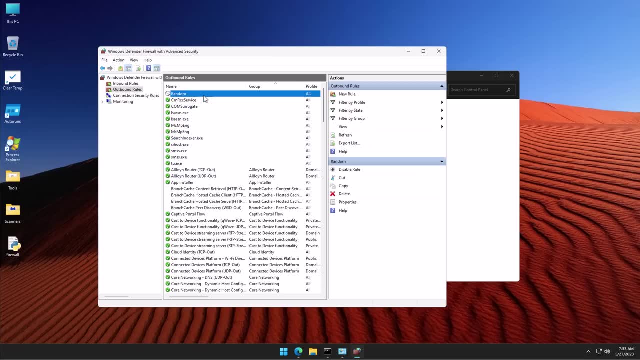 address. So if you type in add and any kind of random IP over here, hit OK. Next you can say block the connection, give it a name and it's done. But that's just one IP and that's not very. 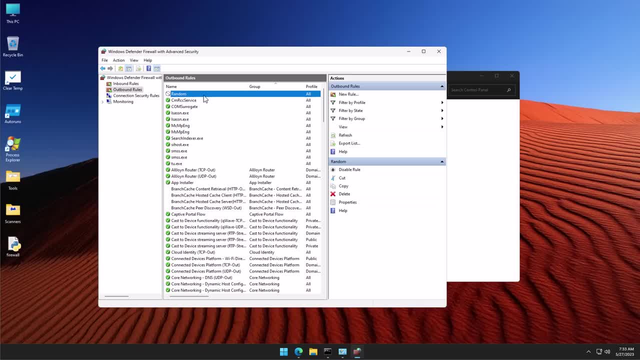 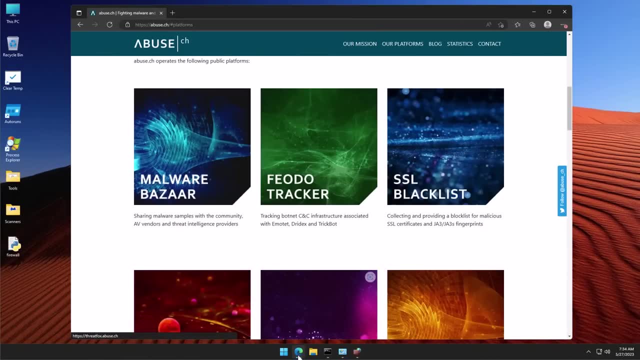 useful. What you want to do is have a list of the most malicious IPs and update that list every day, And that is exactly what I'm going to show you how to do today. So, to start off, how are we going to get this list of malicious IPs? For starters, you could go to abusech and check out. 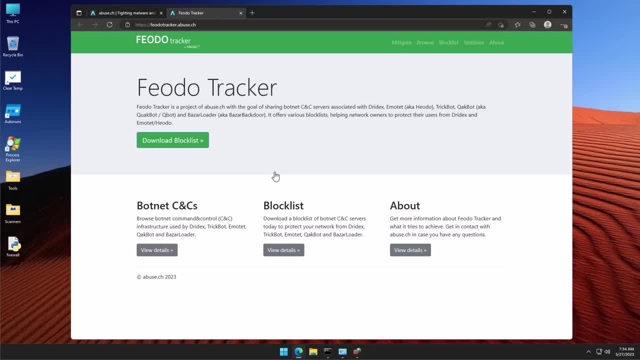 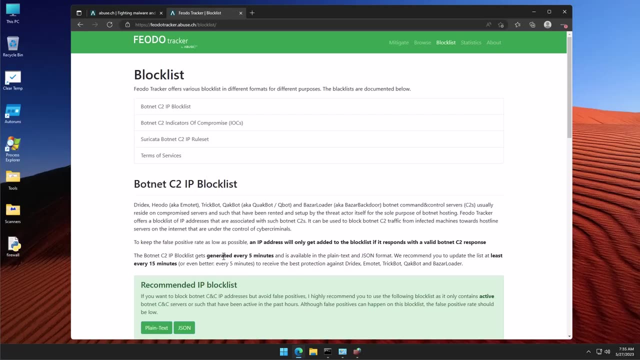 their botnet tracker And this is going to give us a list of bad servers. They're hosting command and control infrastructure for attackers, trick bots, emotat, whatever- And you can actually access this for free And, as you can see, the botnet C2 IP gets generated every five minutes. 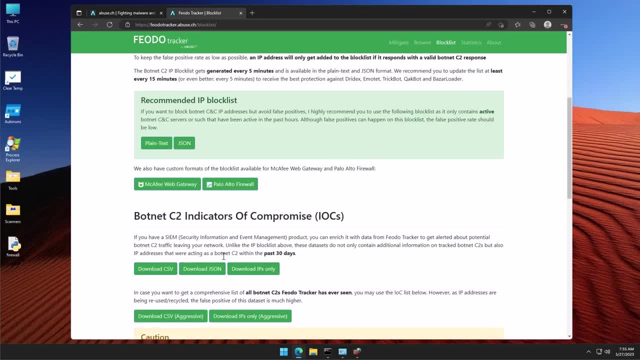 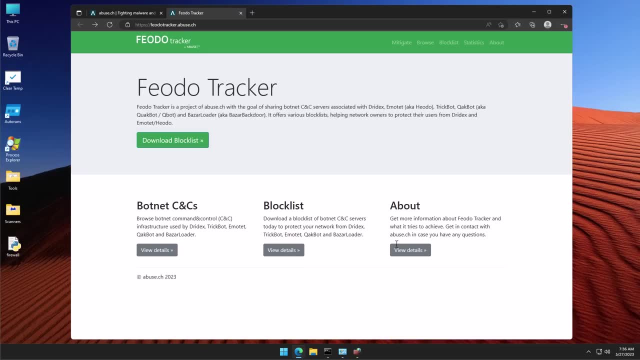 It's available in plain text and JSON. You can also get the indicators of compromise as a CSV. Of course, this is just an example. You can use a variety of approaches, So you could also use this, for example, to blacklist outgoing connections to. 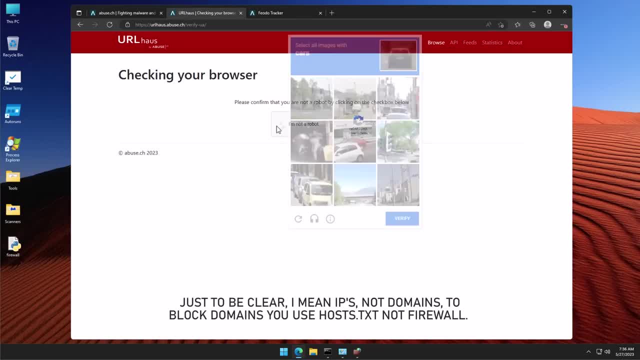 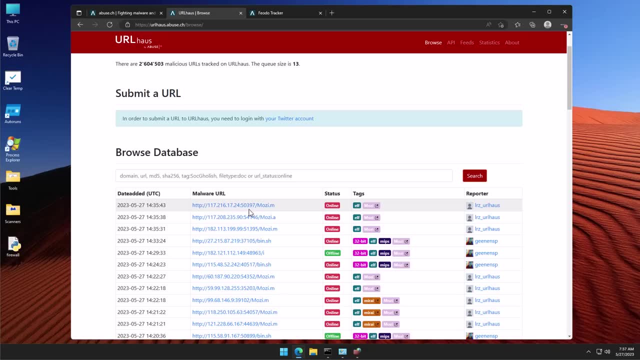 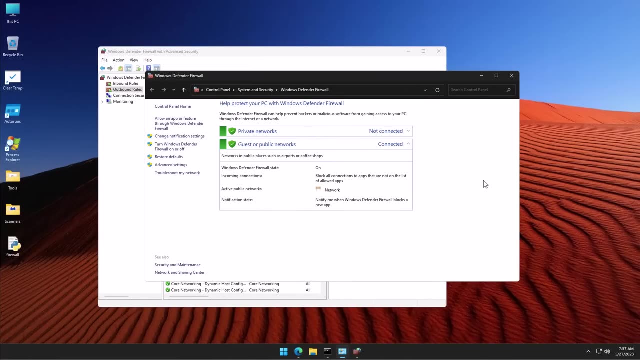 malware domains. So if you go to URL house, for example, you can see a list of malware URLs And again, you could totally blacklist these IPs so that your computer would not be able to connect to them and download the malware. In theory, you could also use it to block Microsoft spying on you. 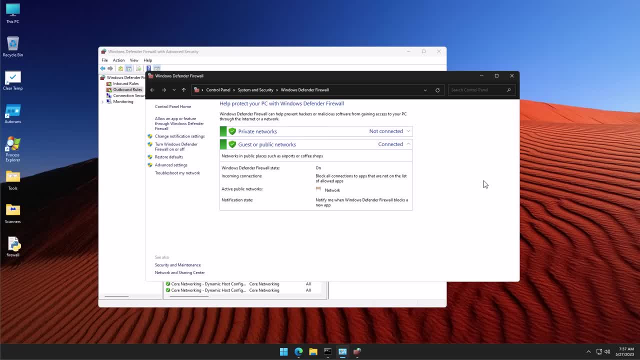 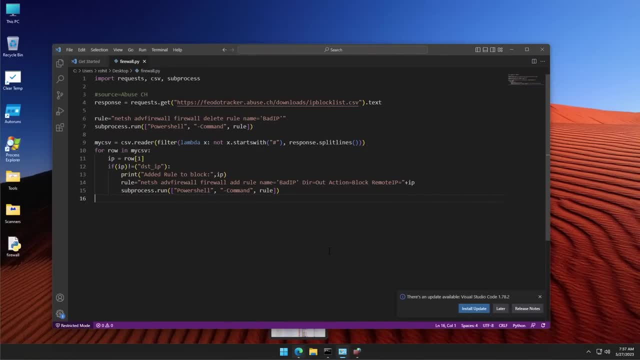 or any other servers you would like to block. The question is, how are you going to automate that and get that list up to date? And if you do, you could also use it to block Microsoft's website every day. Well, actually it's not that hard. As you can see, I've written a very quick 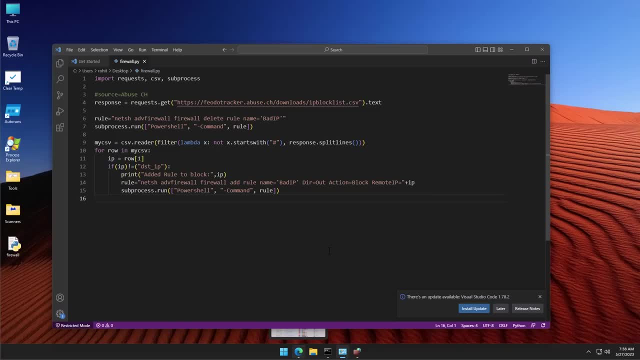 script that's going to do just that, And I'm going to run it and show you how it works. So first we're going to import requests- CSV subprocess. These are just some of the libraries that we're going to use to make our job easier. Then we're basically going to download the CSV file containing 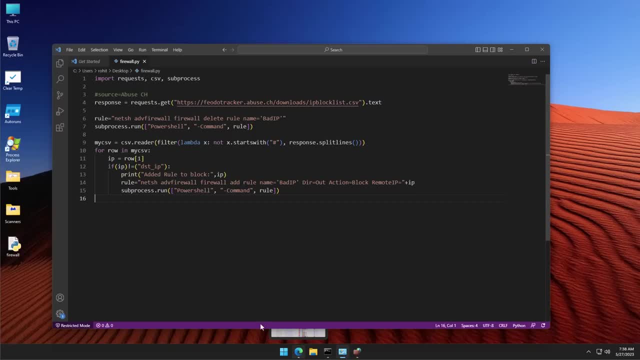 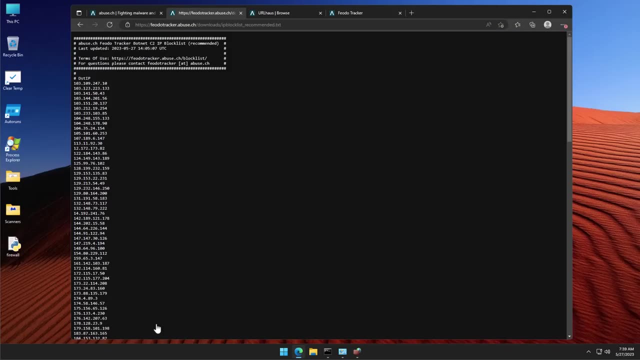 all of the IP addresses. And just so it's not intimidating, I'm going to show you what that actually looks like manually. So if we take a look at the plain text, this is what it looks like. That's literally it. So you've. 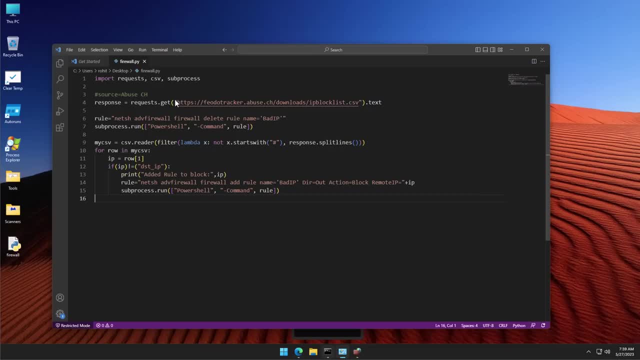 got destination IP and then the IP addresses, and that's it. We're going to grab this file in a CSV format, convert it to text and then just automate typing in a command to add this to Windows Firewall. First of all, though, I'm deleting every rule that already exists with this name. 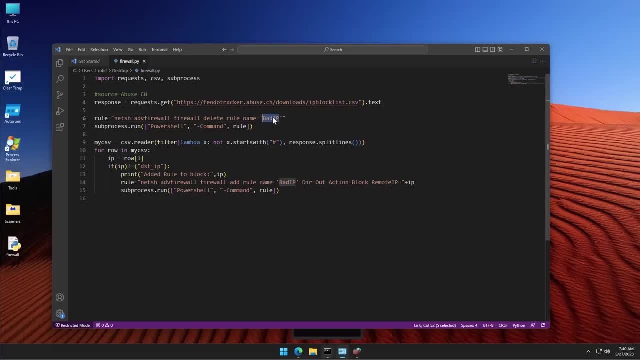 because what we're going to do is we're going to use this name to create rules to block malicious IPs, And I wanted to set it up so that every day it's going to delete everything and then get the new list of IPs, And that's important, because malware IPs don't always stay. 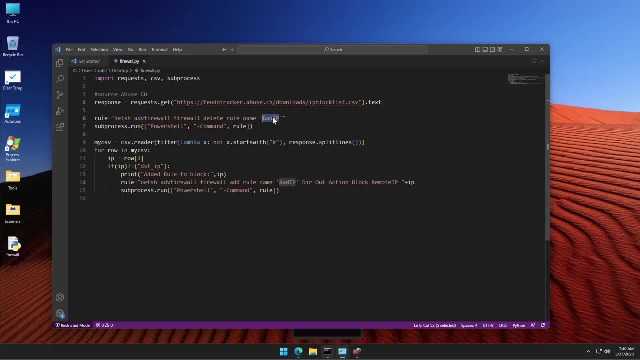 the same. Sometimes an IP may be malicious because the attacker is controlling legitimate infrastructure, So it has to be dynamic. So first we're going to delete everything so that every time the script runs we have a new set of rules and the old rules don't just stay there. We're 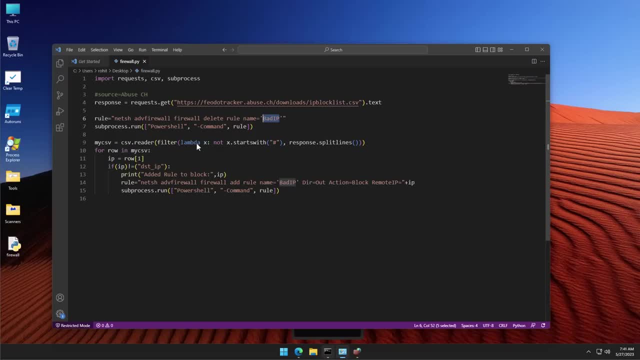 going to use CSV reader, a lambda filter. What this is going to do is basically just filter out lines that do not start with hash, because that is a comment line And if we go back to our actual file, you can see that there is a. 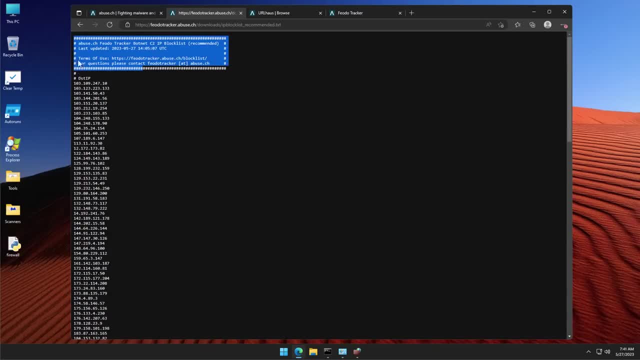 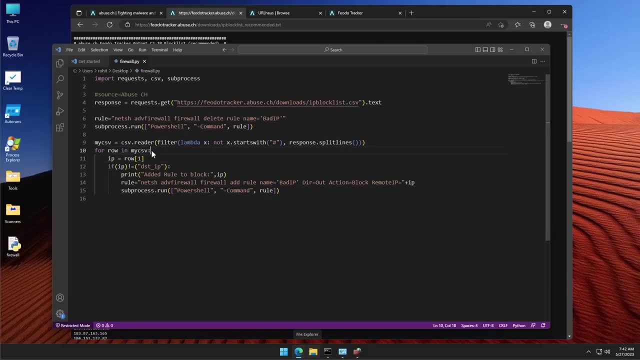 bit of a heading that has the whole hash structure in it, So we don't want these lines to be included in our rules. you kind of want to start from here And then, for each row within that list, we're going to assign the variable IP to row one. that's because of the format of the CSV And 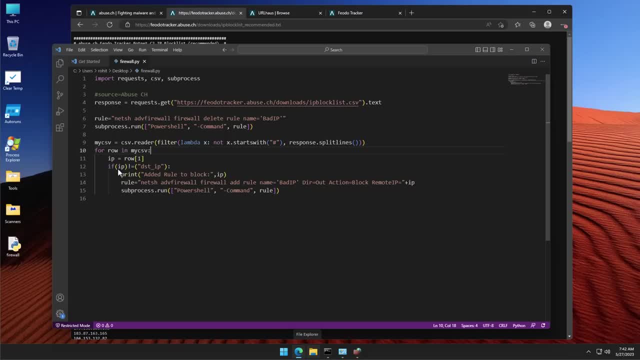 there's some other things that we're going to need to do. So, first of all, we're going to need to add an additional check over here, because sometimes you don't have a hash before the actual column name If the text is not destination IP, which would be the heading of the column. 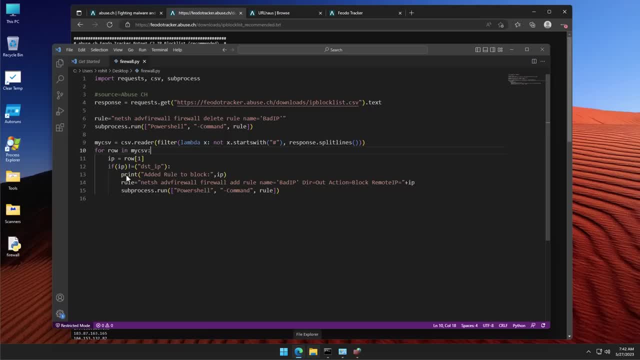 we're going to grab that IP. So all of this is just so over. here in the variable IP we actually have the IP address And then it's just going to print what IP it's going to block. it's going to run a command And this command is basically going to add a rule. call it bad IP. the direction is: 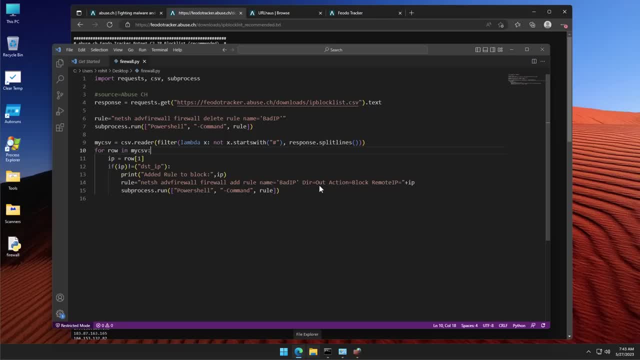 outbound. In this case, we're going to call it bad IP And then we're going to call it bad IP. Obviously you want to add inbound as well if you're trying to block the botnets from connecting to you and prevent things like DDoS attacks. This is just an example. the action is block. 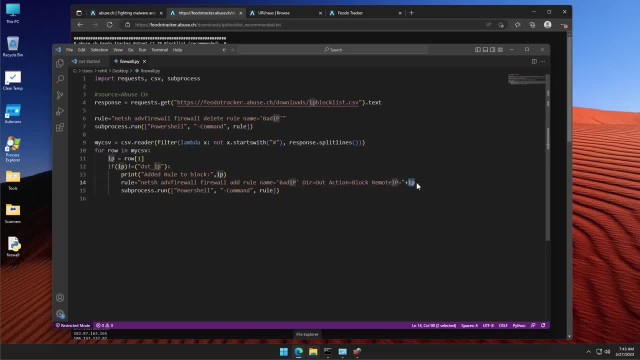 and remote IP equals, and then we're just passing the variable here And then sub process style run. this is just going to run the thing and PowerShell. It's the same as me copying and pasting this command into PowerShell and running it myself, except it's going to do that for every. 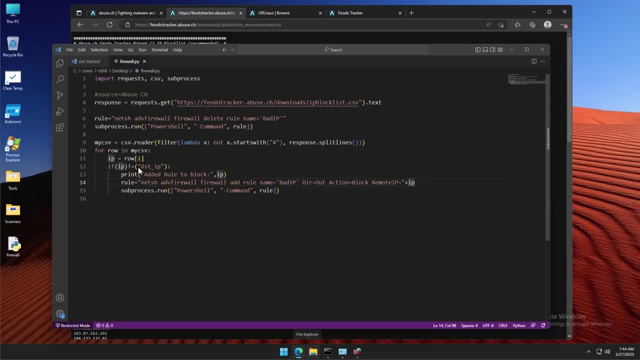 single IP. that's there in the whole list. Pretty straightforward. you could do it whichever way you want. So, for example, you want it to do the same thing but for inbound. you would just copy and paste this And pretty much just change the out to an. 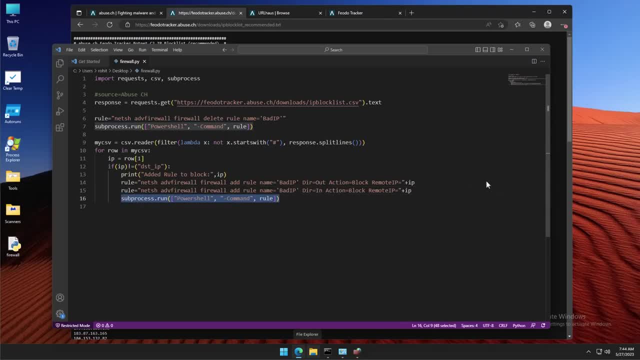 in, And that would do it. you want to do both? then you just copy and paste this here, And now it's running for both. Again just to be clear- though, this is a proof of concept- I'm just trying to show you what you can do with Windows Firewall. you can set it up however it makes. 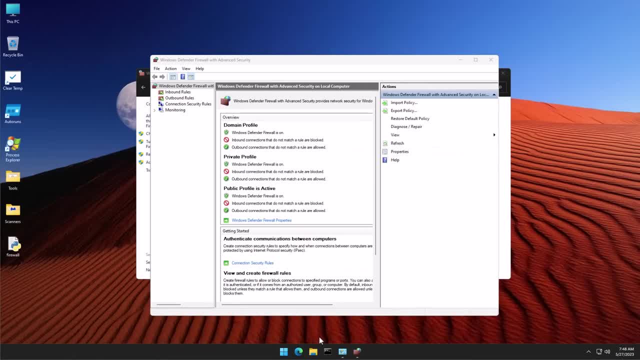 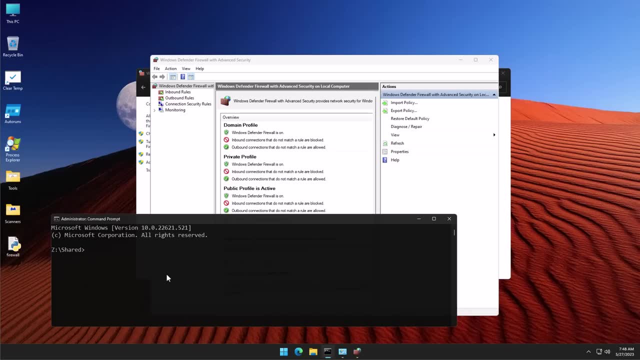 sense in your environment. Now all that's out of the way. let's see it in action. So I'm just going to open up regular command prompt. Remember, you have to do this as an administrator, just going to drag my script in, we're going to run it And hopefully that's going to add rules for each. 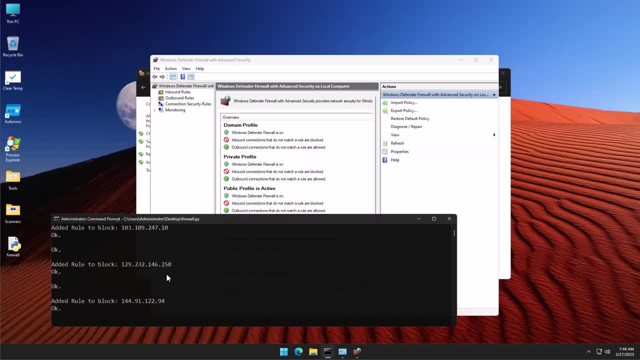 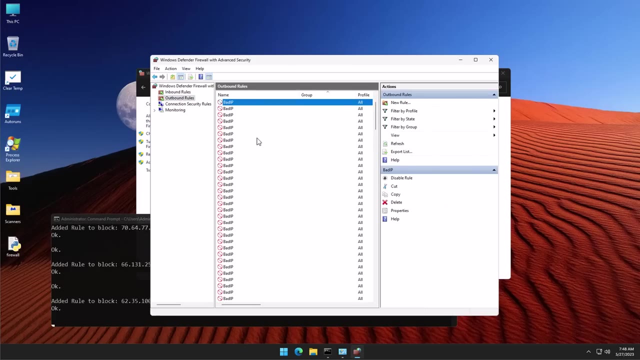 of these IPs. As you can see, it is displaying that on the screen. all of the IPs are being added one by one And once the script completes, all of those rules are going to be in here And we can check that it's doing that. So you can see, for the outbound, we do have a lot of. 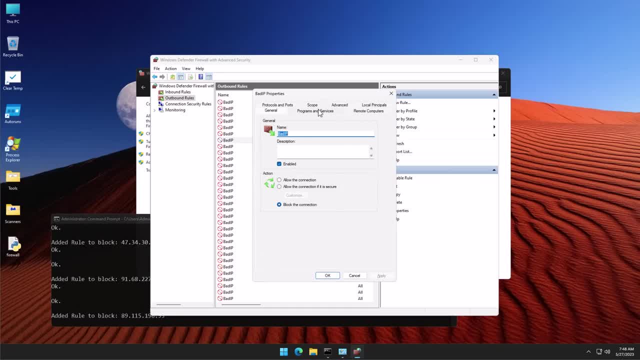 bad IP rules already, And if you open it, you're going to see that the scope says that these IP addresses which we've got from our block list derived from abuse reports, open source threat Intel, and now we're actively blocking it on our system. you can, of course, use a similar workflow. 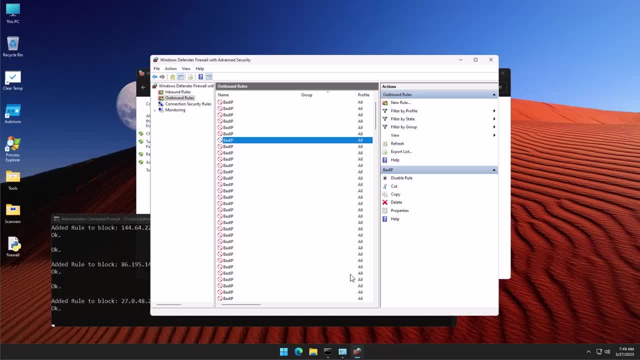 for any kind of firewall software, regardless of whether or not it's Windows Firewall, third party firewall. typically good third parties will have that built in. So they're going to see a lot of bad IPs and they're going to want to subscribe to a certain block list. But as far as 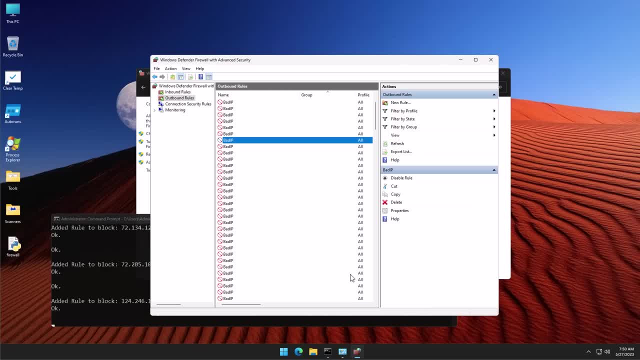 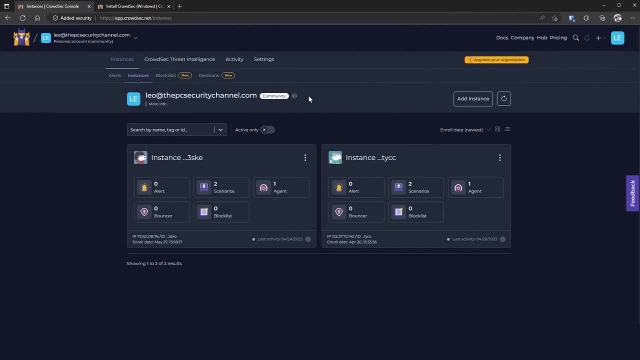 I'm aware I've never really seen Windows Firewall block the IPs- the malware IPs I test with, So it may be a good exercise, especially if you're running some kind of server. Now, an extension to what we just did would be to use something like Crowdsack, which is an open source intrusion. 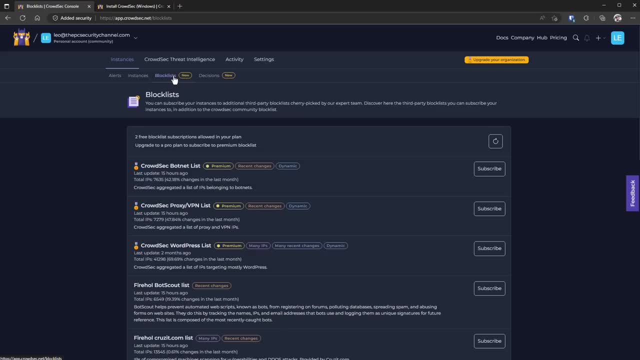 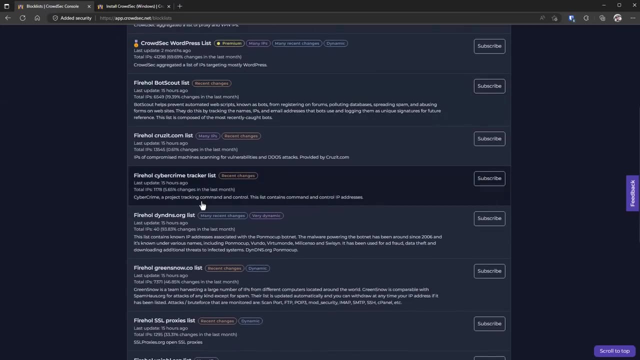 detection system and also the sponsor of this video. It's cross platform, so you can install it on Windows or Linux And then, if you go into block lists, you pretty much have a list of block lists that you can just subscribe to, So you don't have to manually go in, find a way to 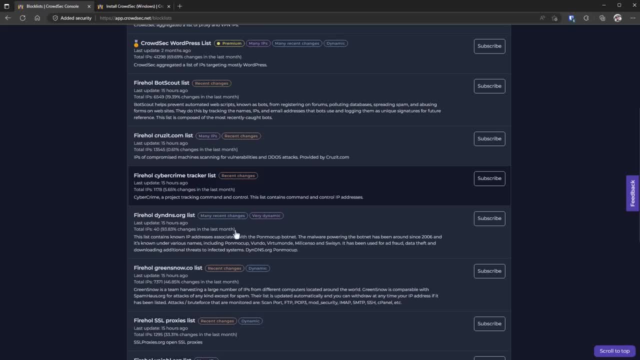 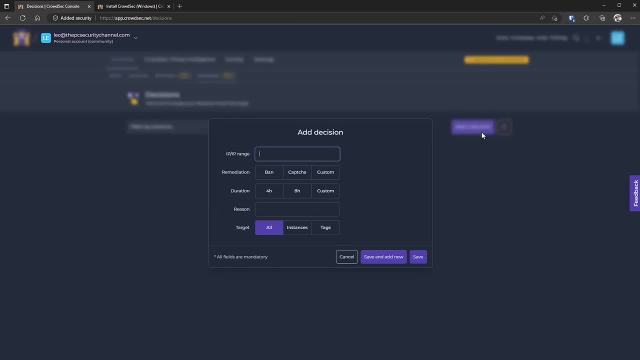 automate the integration of that. all of that work is done for you. you just click on the subscribe button and you just get a certain block list. There are some free ones, there are some that are premium. you've also got the ability to add custom decisions, which is kind of like a rule, And you 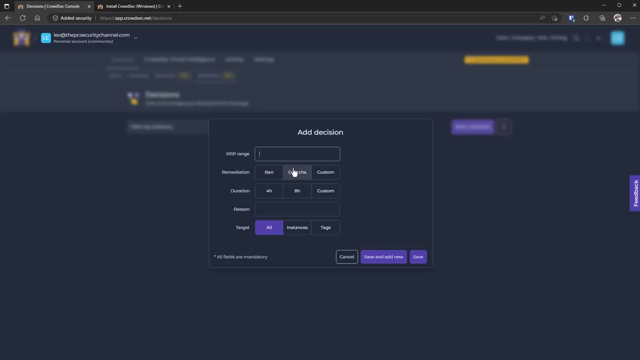 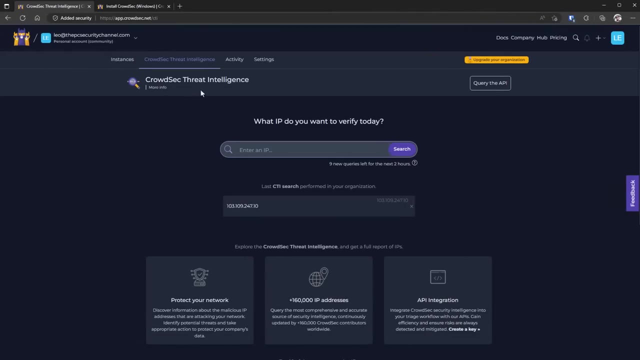 can even add a captcha. So if you're hosting something, instead of just banning an IP, you can just force a captcha for an IP, and then you can select a duration as well. You've also got the ability to add a time limit, which is a little bit more than you would expect. So if you want to, 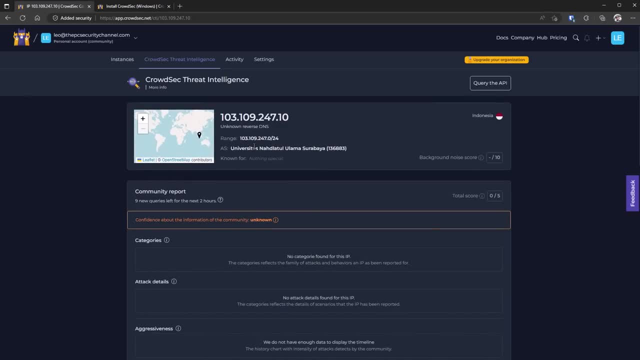 check if an IP is safe or not. you can just type it in and it's going to tell you where it's located. what the community reports are- you can see how many queries were made in the last two hours. In this case, based on all the information, the confidence about this is unknown, but it can tell. 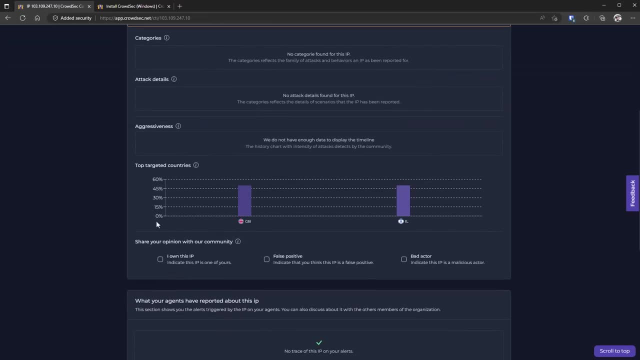 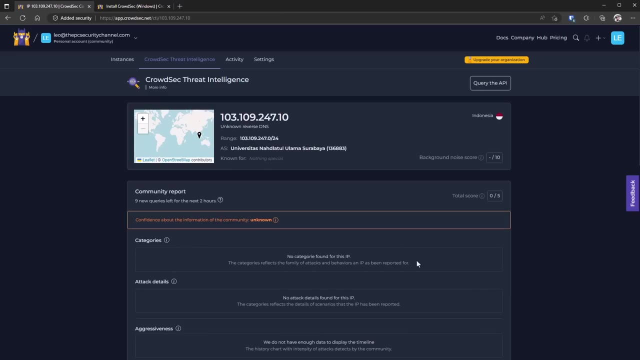 you. if something is certainly malicious, For example, it's all community based, so you can vote on it yourself. You can say if it's your IP, if it's false, positive or if it is malware. It's crowdsourced security, so it's not necessarily a threat to the IP, but it's a threat to the IP.